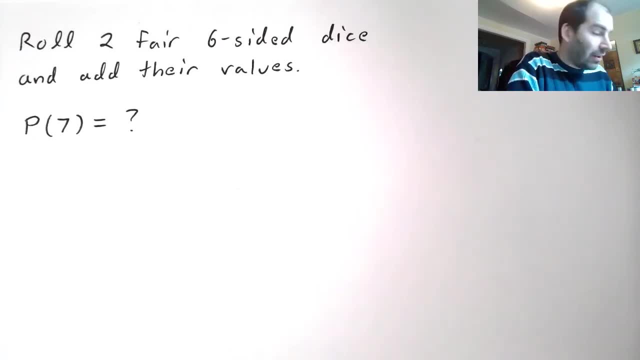 The naive approach would be to list the sample space as follows. Here's our sample space, all possible outcomes. Well, when I roll two six-sided dice, the smallest number I can get is a two. I can roll two ones. I could get a three by rolling a one and a two. I 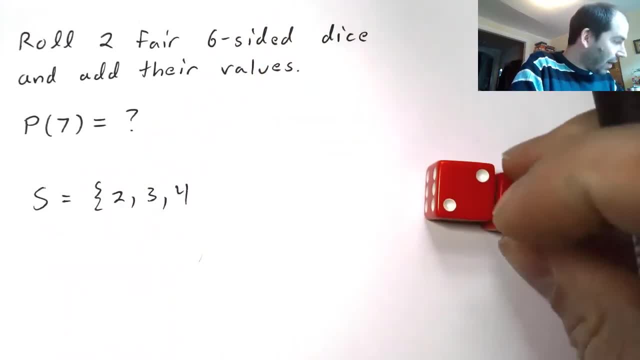 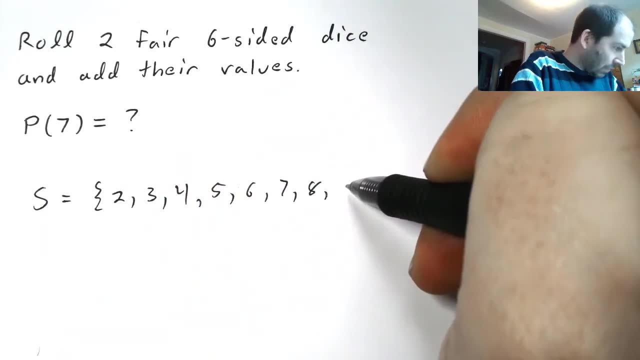 could get a four by rolling two twos. I could get a five by rolling a two and a three, etc. I can roll all kinds of numbers here, And the largest number I can get is a 12, because I can roll a six. 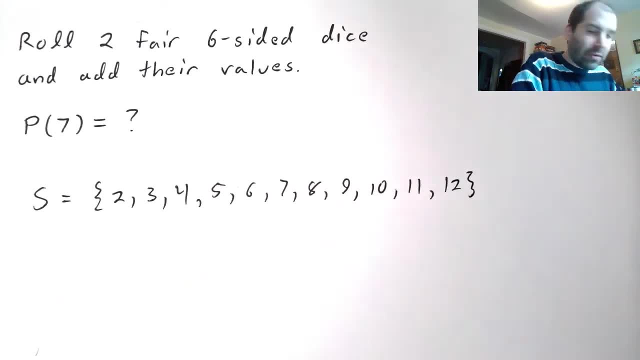 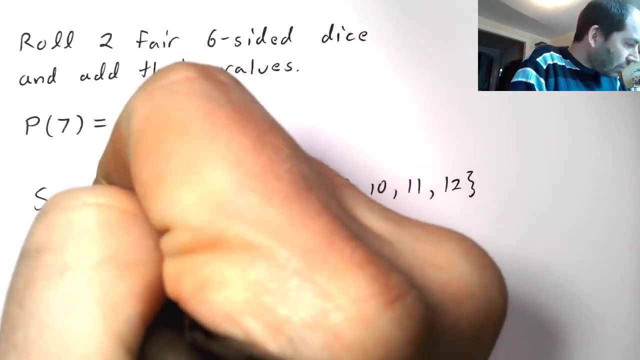 So these are all possible outcomes, And in the previous video we talked about one mistake that someone might make is might say: well, the probability of getting a seven. to compute that. what I'll do is: I'll see how many of these things equal seven. Well, 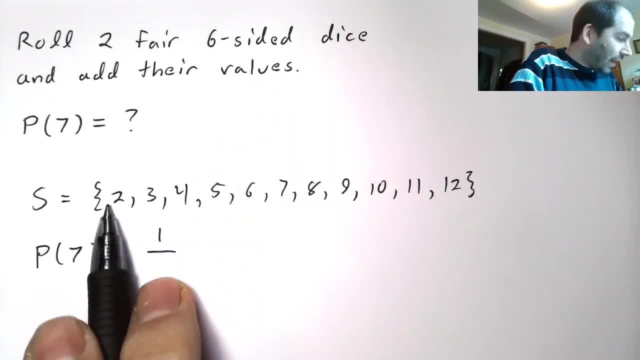 only one of them, Count one, and then I divide by the number of things in the sample space: One, two, three, four, five, six, seven, eight, nine, ten, eleven, twelve, thirteen, eighteen, nineteen, twenty, twenty-two, twenty-three, twenty-four, twenty-five, twenty-six, twenty-seven, 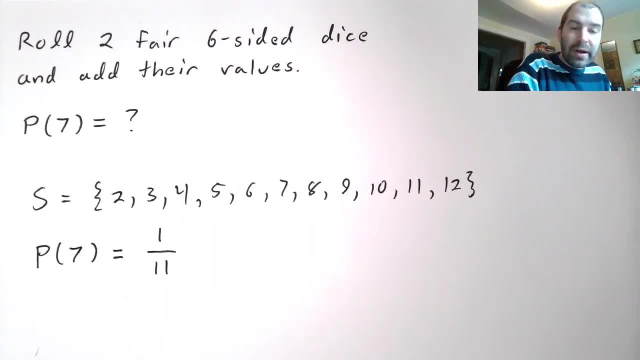 twenty-eight, twenty-seven, twenty-eight, twenty-nine, twenty-eight, twenty-nine, twenty-ten, twenty-eleven, And I might think that this is my answer, but we discussed how this is not the right answer. And the reason that's not the right answer is because the method 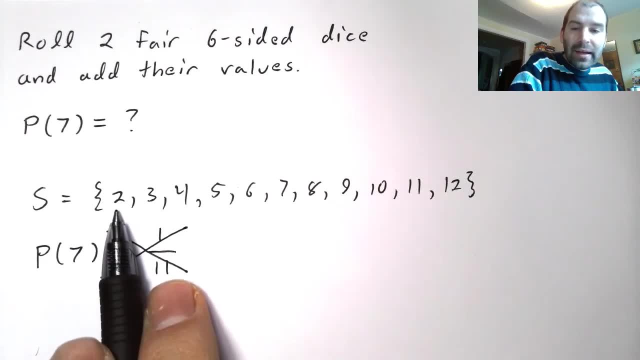 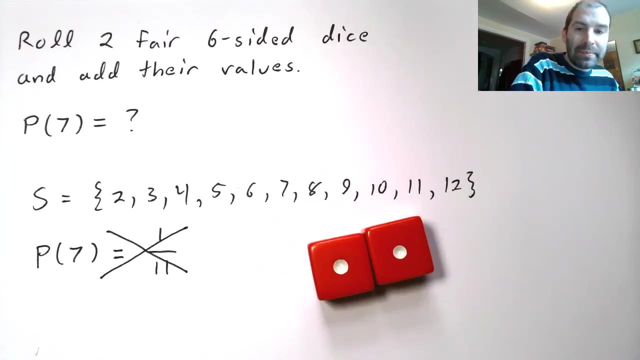 that we're using here depends on all these outcomes being equally likely. But they're not equally likely. For instance, how many ways can I roll a two? Well, the only way I can get a two is by rolling a one and a one. There's only one way that can happen. 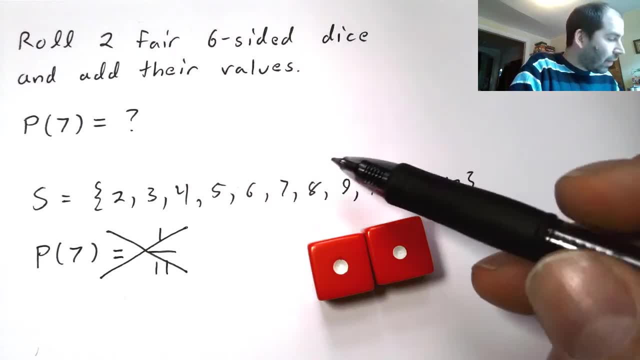 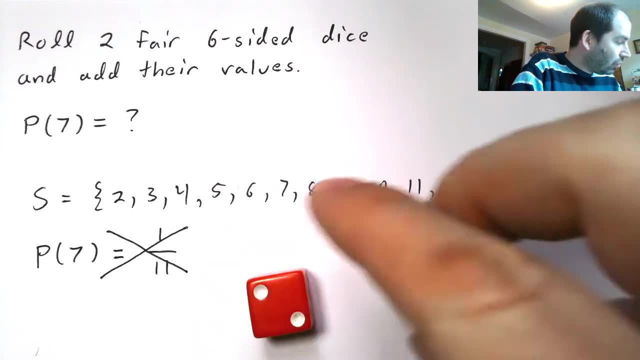 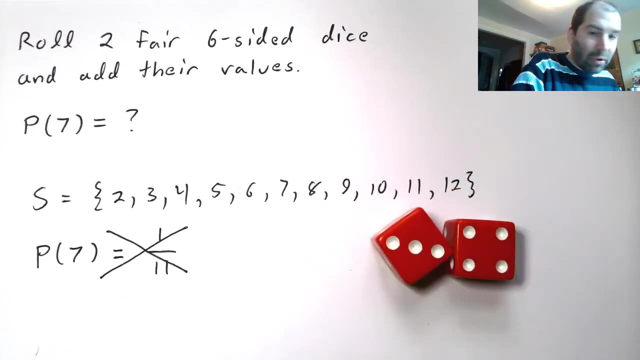 A two is not very likely. However, how many ways can I roll a seven? Well, I could roll a one and a six. I could roll a two and a five. I could roll a three and a four. There's several ways to roll a seven, but there's only one way to roll a two. So these can't. 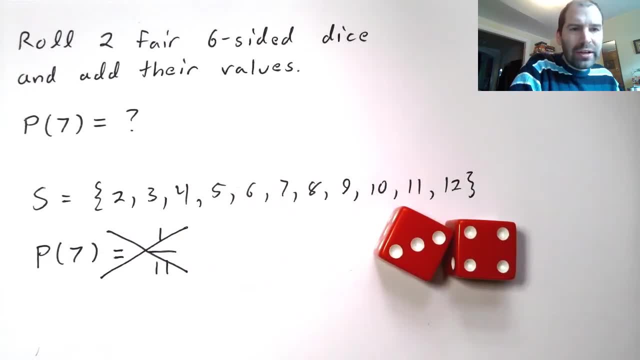 be equally likely. Seven, for instance, is more likely than two. So we can't use that rule that got us one over eleven. That rule is not guaranteed to get us the right answer. So what we need to do is we need to view the sample space in. 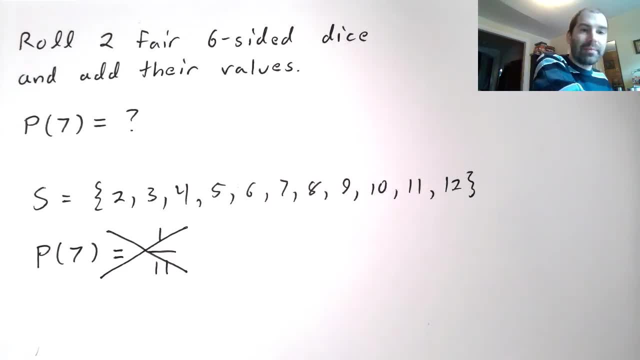 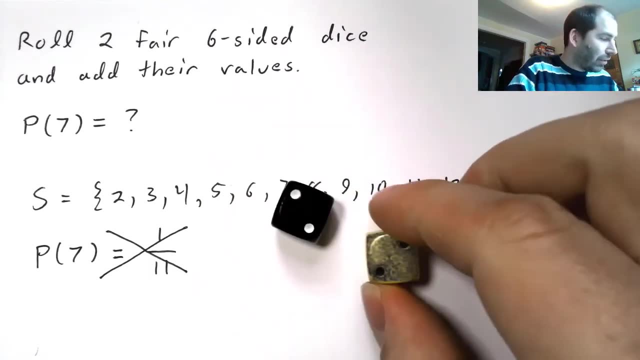 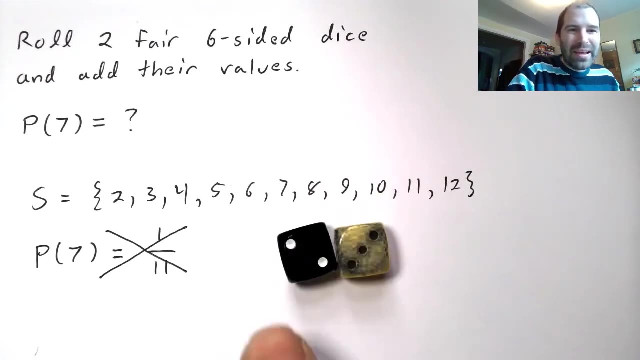 a different way. So this is the trick for this problem, And the way we're going to do this is we're going to imagine that we have two differently colored dice. Oh boy, this one is not showing up very well on my green screen because it's a green die, But anyway. 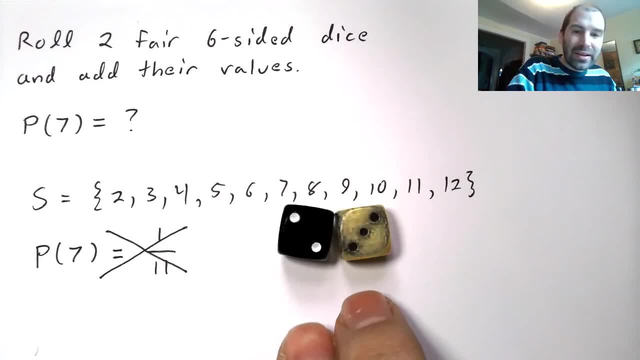 you get the idea. There's two differently colored dice, And so if we think of the dice this way, we can imagine the sample space a little bit differently. So what I'm going to do is I'm going to depict each die's value separately in a table. So let's go ahead and 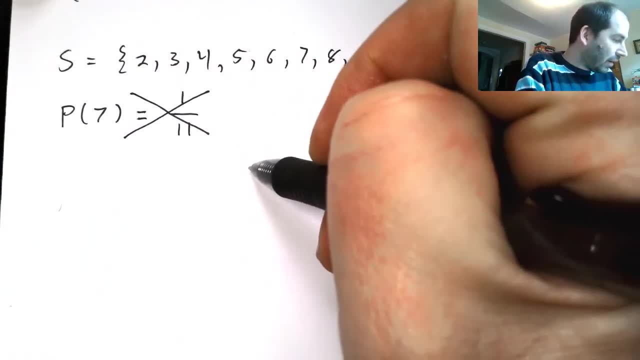 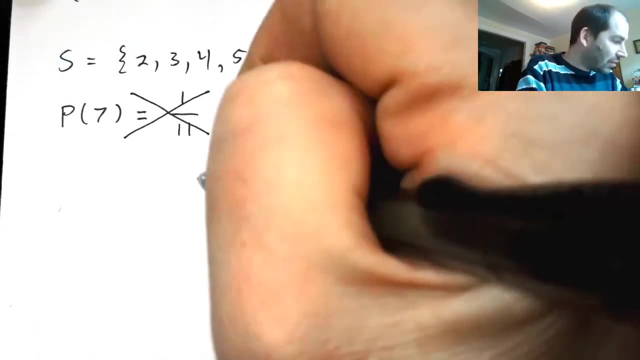 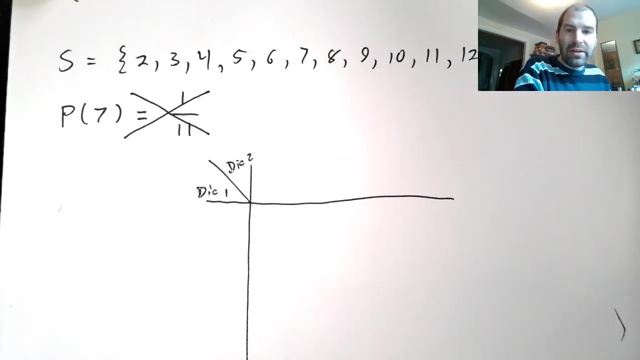 write this table out. So we're going to have the columns of the table representing the value of one die, And so we'll call that die1.. And then the rows representing the values of another die. I think I said that backwards, So the rows are going to be die1 and the columns will be die2.. So what are the values I can? 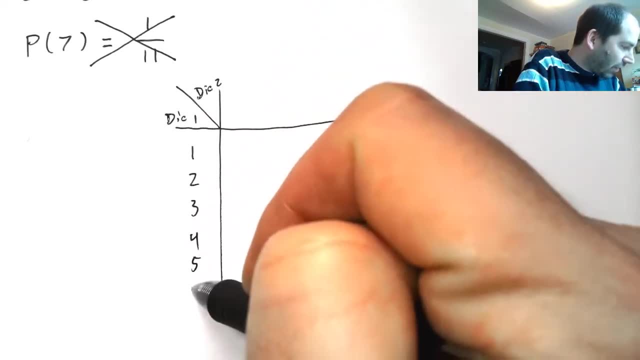 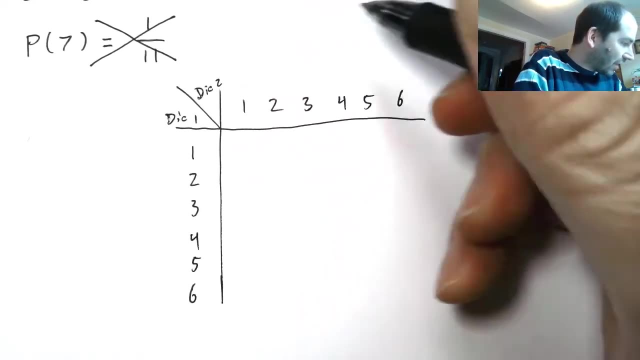 get for die1?? Well, I can get 1,, 2,, 3,, 4,, 5, or 6.. What are the values I can get for die2?? Well, 1,, 2,, 3,, 4,, 5, or 6.. 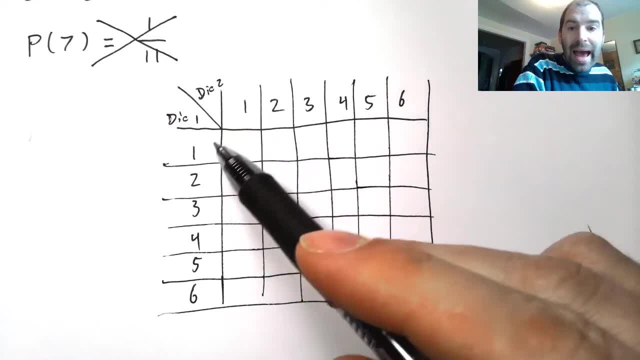 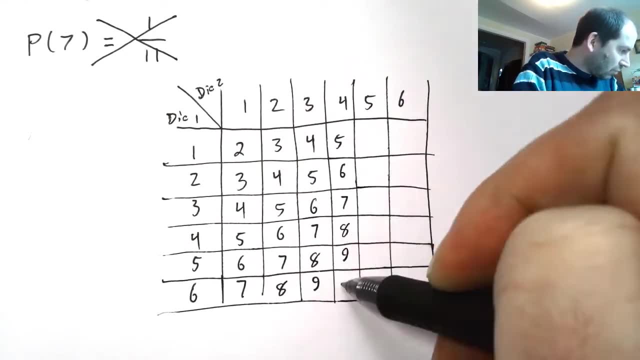 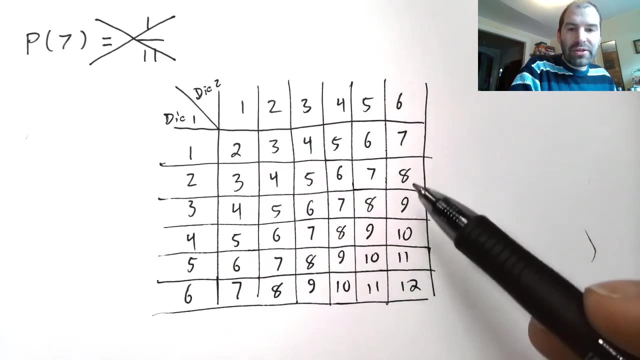 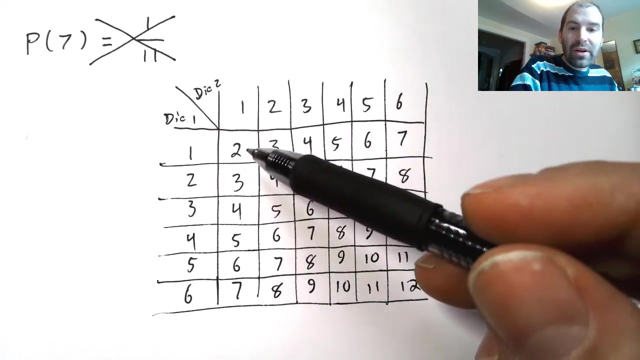 Okay, Let's fill in this table by adding the values of the dice, because that's what we're doing in this experiment. Okay, So I have written inside the table the sum of the two die values. I've added them together. Now what I'd like you to observe is that each outcome in this table is just 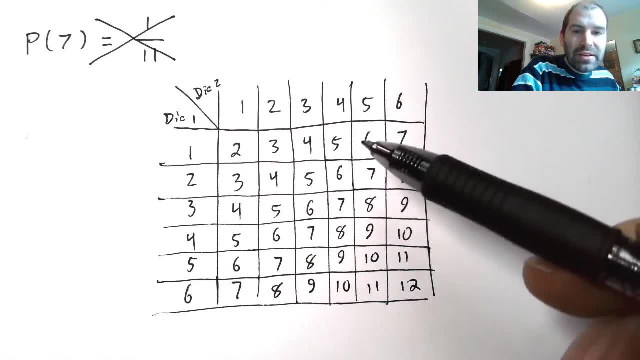 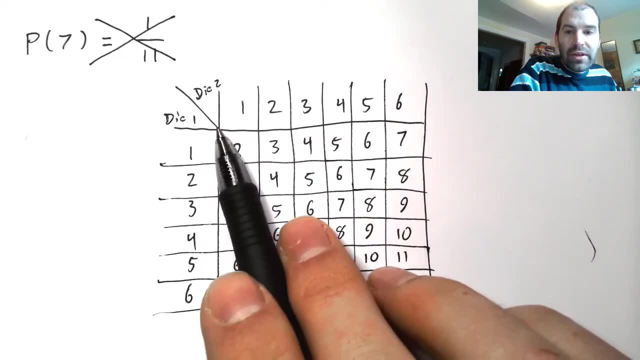 as likely as any other outcome in this table. Okay, these outcomes are equally likely. Why is that? Well, because these are all equally likely. These are all equally likely. So a combination, a given combination of them, say a four and a three. 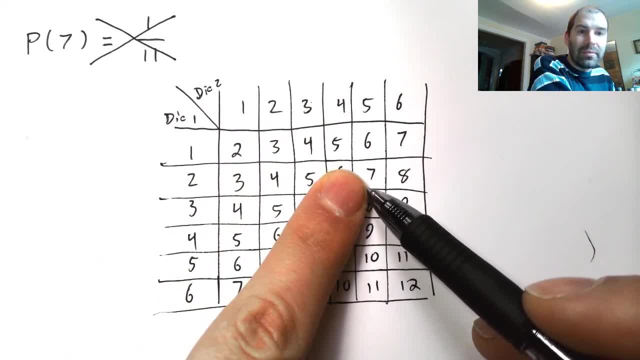 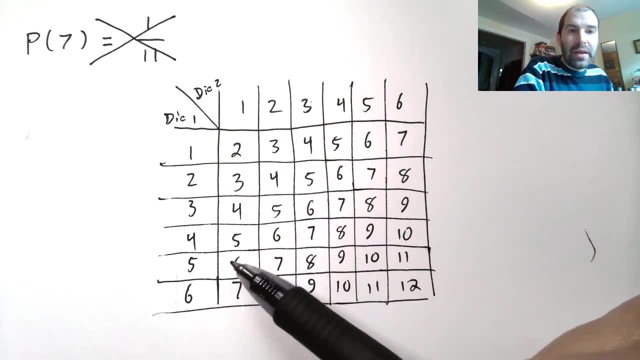 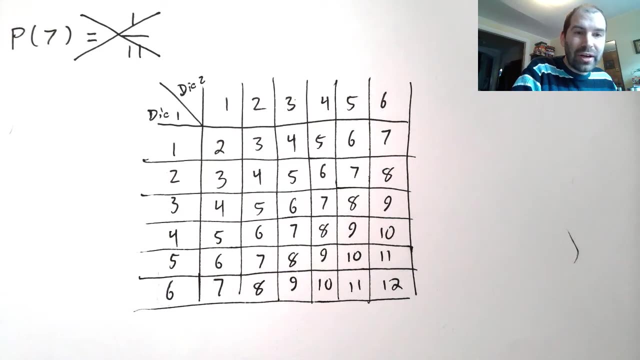 is just as likely as any other single combination of them. So these outcomes inside the table are all equally likely. So now that we have a sample space of outcomes that are equally likely, we can use the approach that we tried before, using this as our sample space.